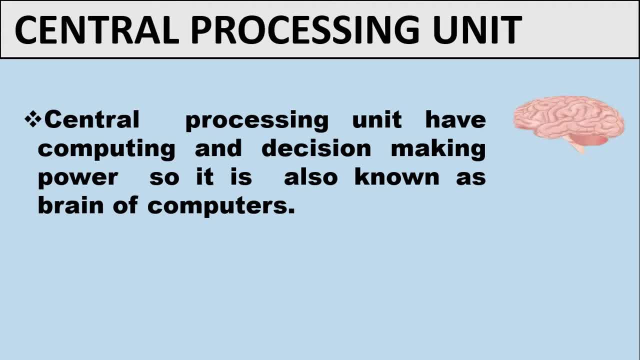 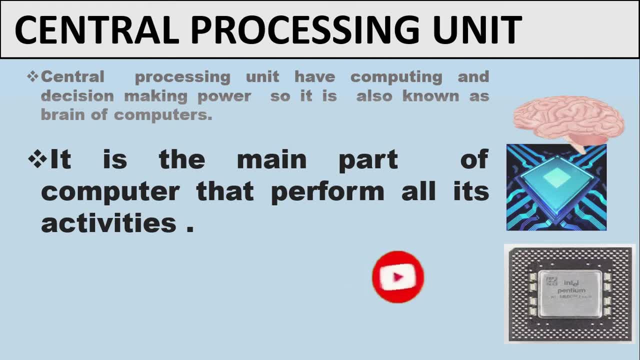 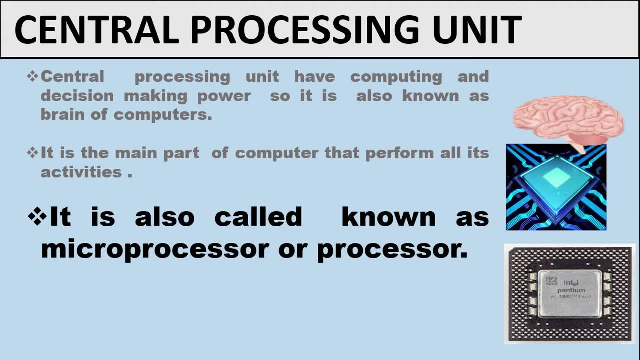 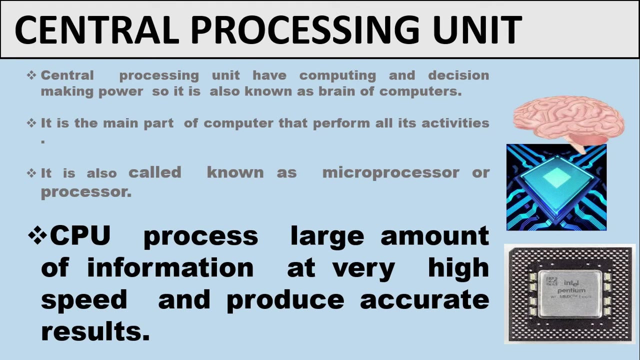 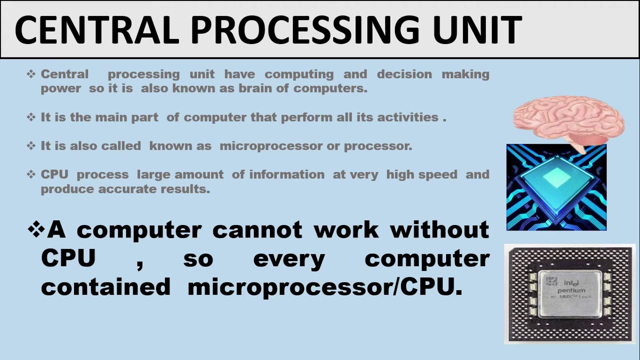 So it is also known as computer. It is the main part of computer that perform all of its activities. CPU is also known as microprocessor or processor. CPU process large amount of information at very high speed and produce accurate results. A computer cannot work without CPU. 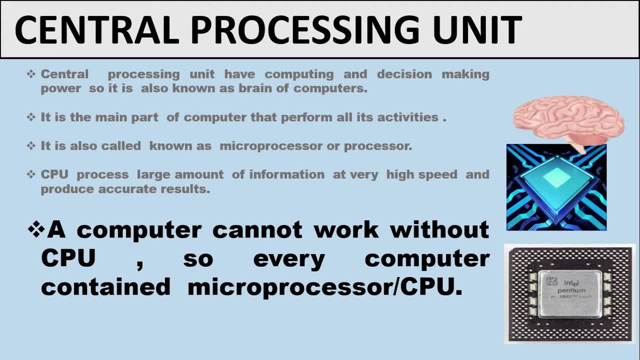 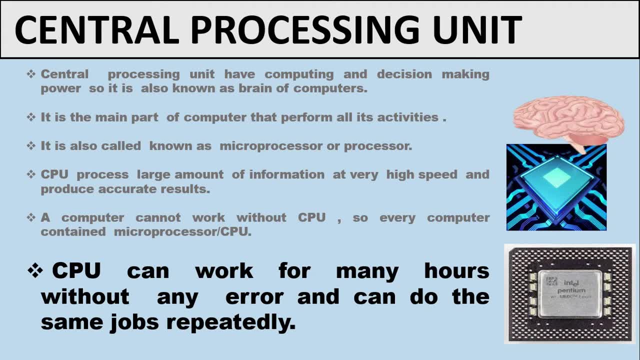 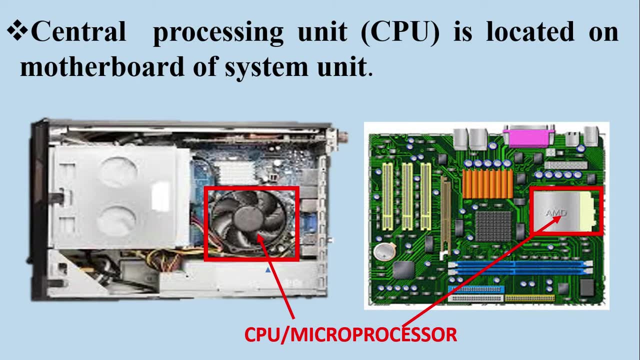 So every computer contains microprocessor. CPU can work for many hours without any error and can do the same job repeatedly. Central processing unit is located on motherboard of system unit. It is highlighted by red square. CPU components are earth, metal, arithmetic and logic unit. 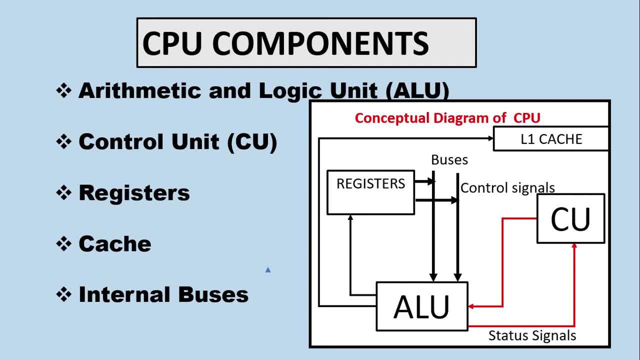 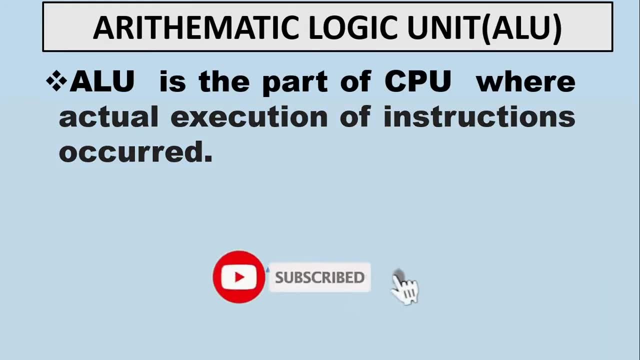 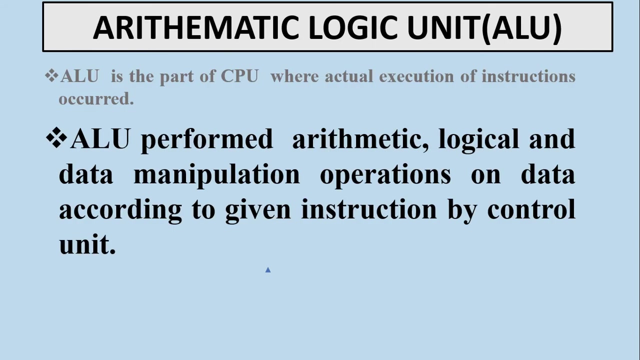 control unit registers, cache memory and internal buses. On the right side is the conceptual diagram of central processing unit. Arithmetic logic unit is the part of central processing unit where actual execution of instructions occurred. ALU perform arithmetic, logical and data manipulation operations on data according to given instruction by control unit. 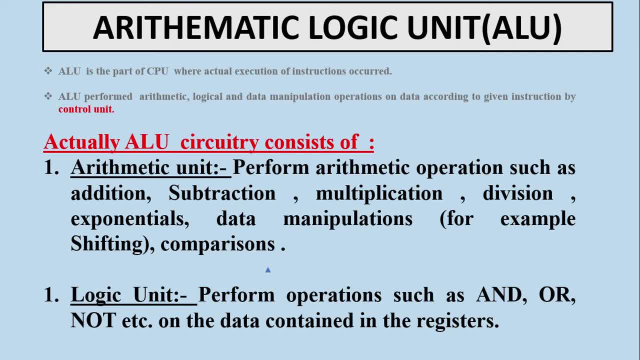 Actually ALU circuitry consists of two units: arithmetic unit and logic unit. In arithmetic unit, ALU perform addition, subtraction, multiplication, division, exponential and data manipulation, for example shifting and comparisons. And in logic circuitry, ALU perform and or not on the data contained in registers. 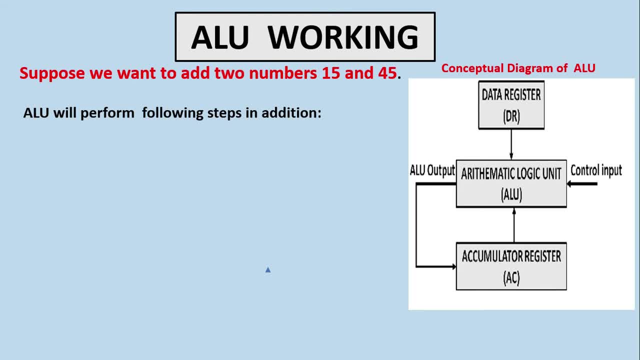 ALU working. Suppose we want to add two numbers, 15 and 45.. ALU will perform following steps in addition: The first number, 15, will store in accumulator register. The second number, 45, will store in data register. Control unit will send command to add these numbers through control input. 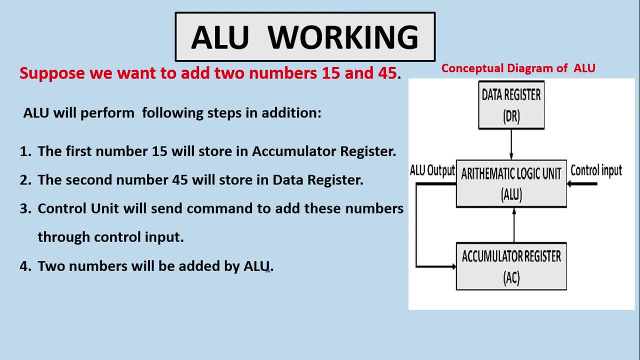 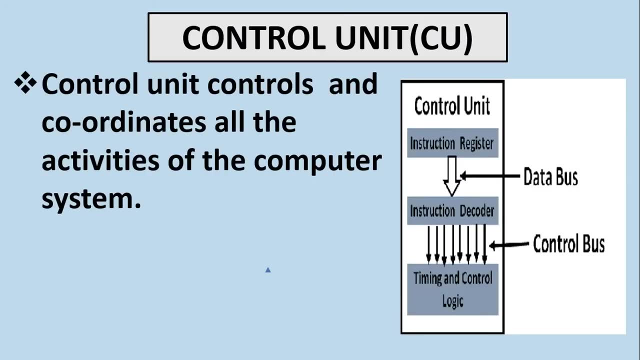 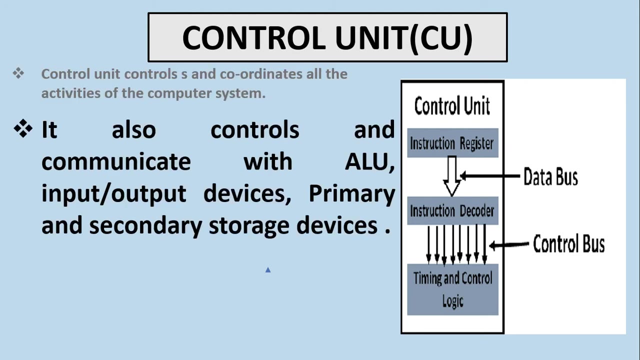 Two numbers will be added. ALU will be added by arithmetic logic unit. The output will be stored in accumulator registers. Finally, result 60 will be sent to main memory Control unit. Control unit controls and coordinates all the activities of computer system. It also controls and communicates with arithmetic logic unit. input output devices: primary. 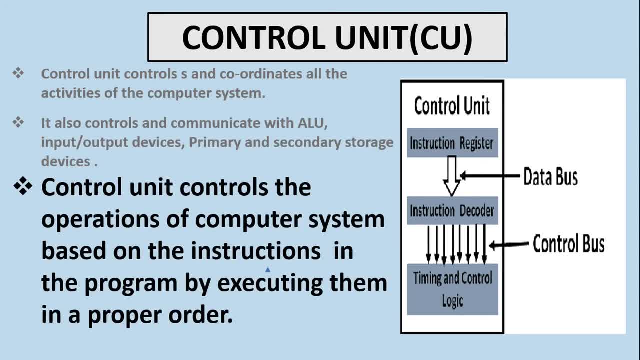 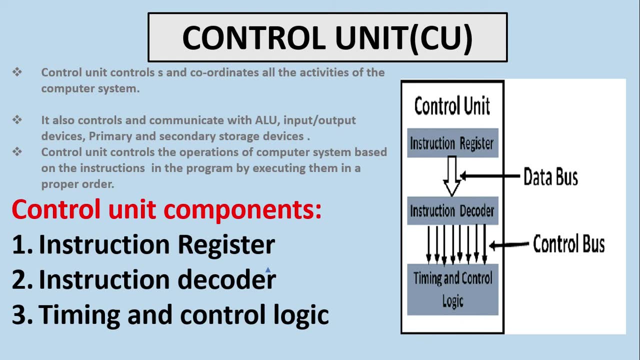 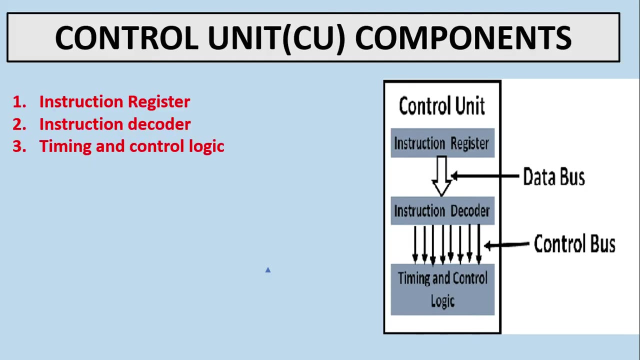 and secondary storage devices. Control unit controls the operation of computer system based on the instruction in the program, by executing them in a proper order. Following are the components of control unit: Instruction register, Instruction decoder, Timing and control logic. Instruction register stores the instruction while it is being executed. 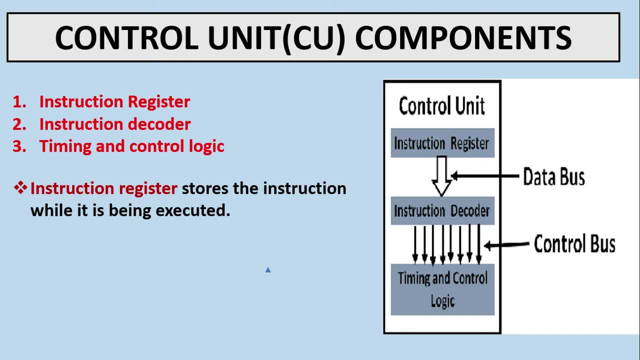 By database. it will go to instruction decoder. Instruction decoder will translate it in binary form. Timing and control logic generate the signals to execute it. Registers: Registers are small, high-speed and complex. registers Analyze the system and the software's software. 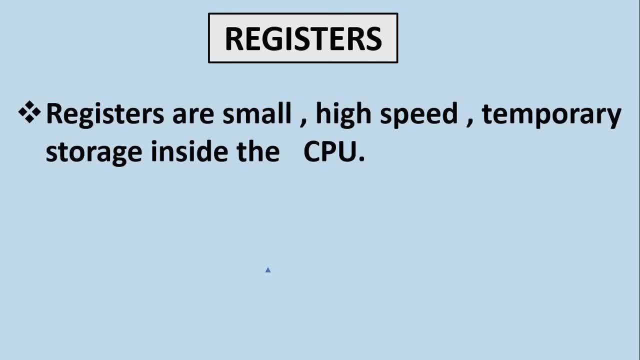 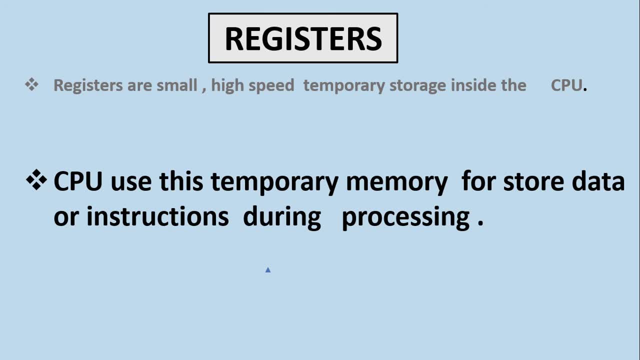 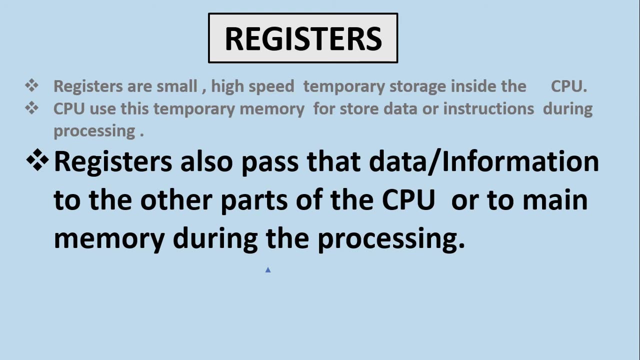 Test, Timing and control logic. The CPU uses this temporary memory for stored data or instructions during processing. Registers also pass that data information to the other part of the CPU or to main memory during the processing. CPU contains several registers. Each register contains a data register. 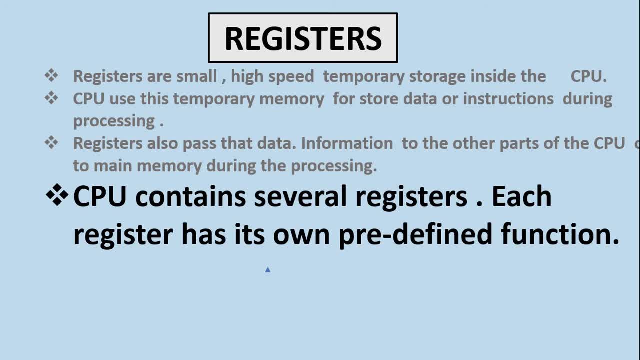 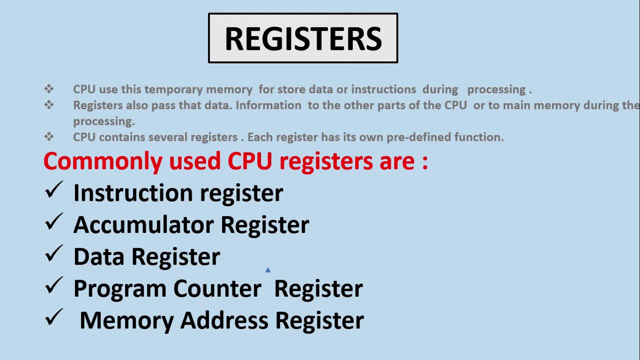 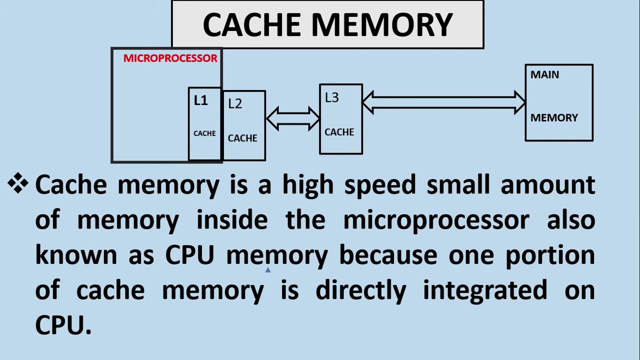 Each register contains a data register Be the computer. The computer has its own predefined function. commonly used CPU registers are instruction register, accumulator register, data register, program counter register and memory address register. cache memory is a high-speed, small amount of memory inside the microprocessor, also known as CPU memory because one portion of cache.